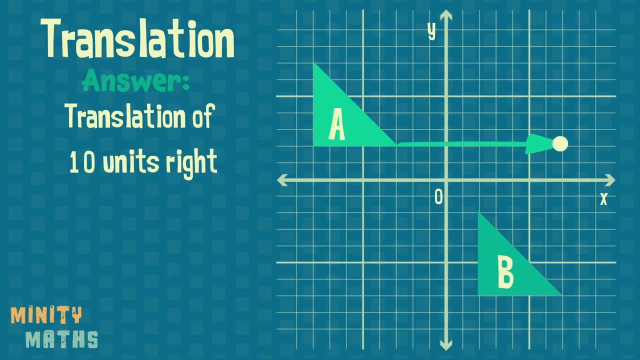 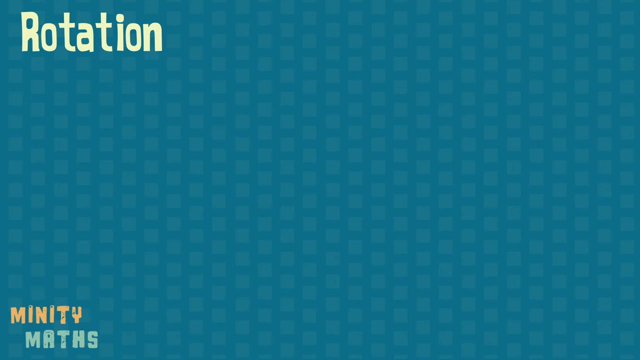 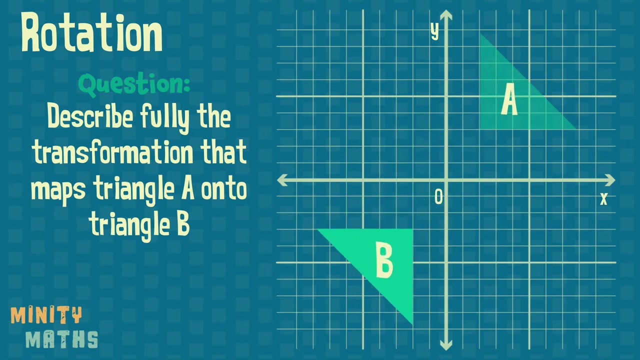 change vertically. Pick any vertex of the shape and use this to count how many units the shape has moved horizontally and vertically. We can also use vectors to describe translations. Translation also changes the shape's position. To describe rotation, we must provide three details. 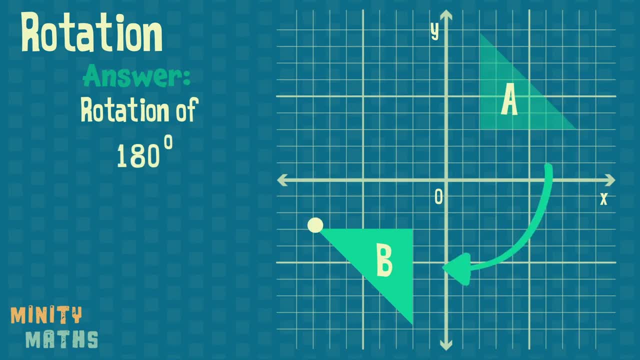 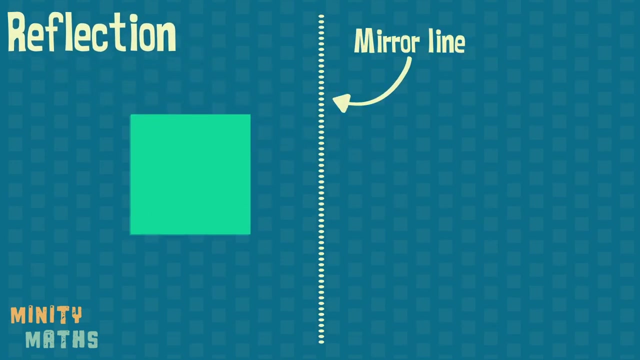 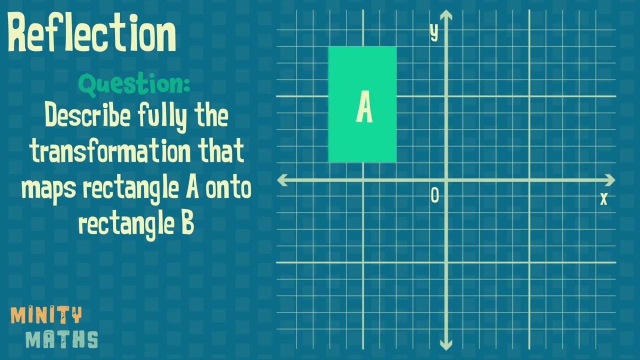 The angle of rotation, the direction and finally, the centre of rotation. You may find tracing paper helps with finding the point that the shape has been rotated. Reflection changes the shape's position. Reflection of a shape can be described using only one detail, The equation of the line. 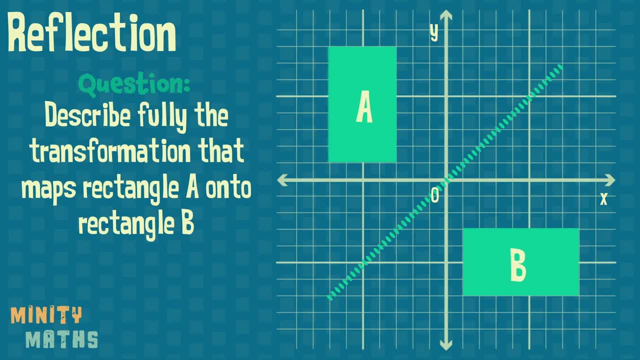 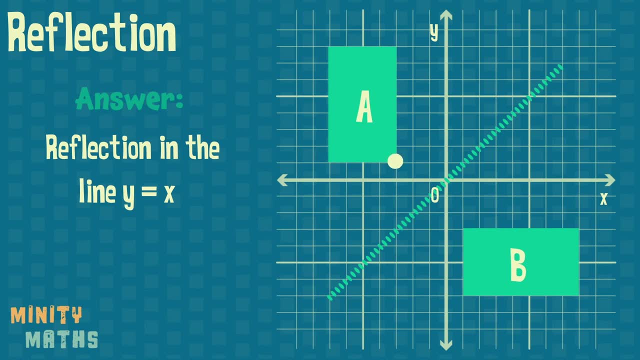 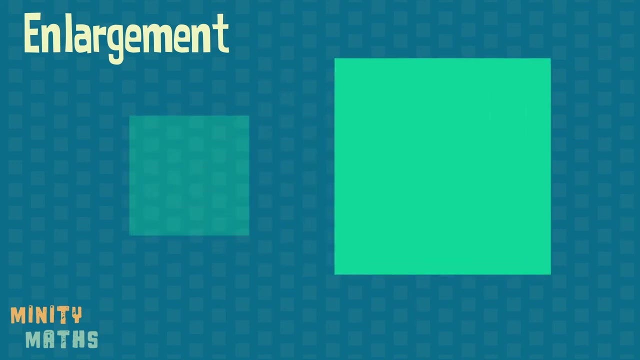 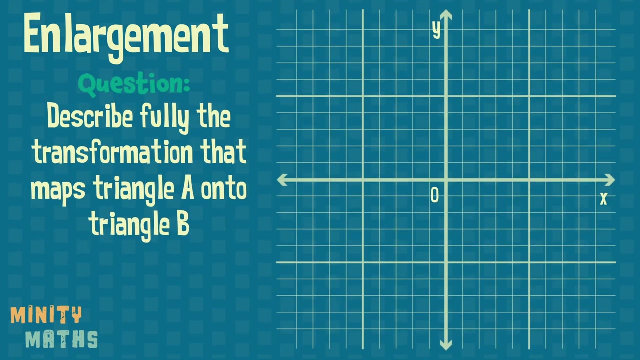 of reflection. It can help to think of this line as a mirror. Each vertex of the new shape will be an equal distance from the previous one. Finally, enlargement changes the shape's size. To describe an enlargement we need two details: The scale factor and the centre of enlargement. 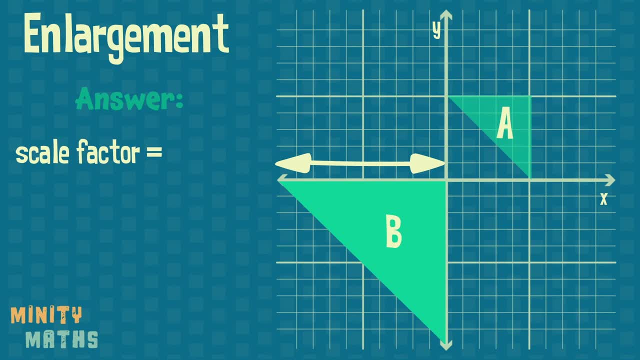 We can find the scale factor by measuring the length of one side of both the new and old shapes. We can then divide the new length by the old length To find the centre of enlargement. draw lines from the corresponding vertices of the new shape and old shape, extending them until they cross. 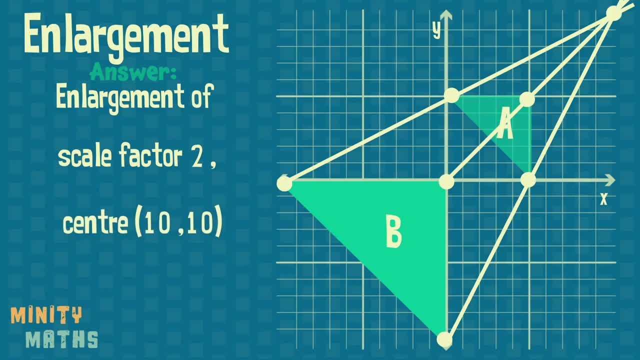 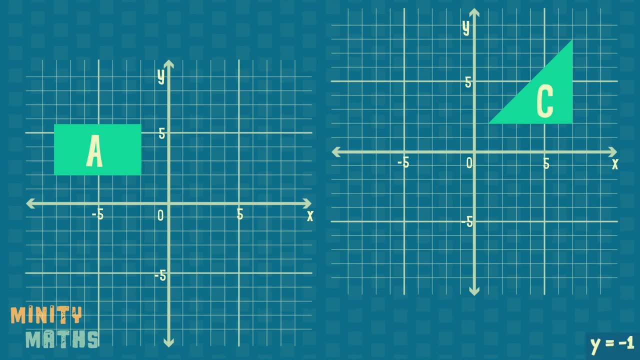 The point at which they cross is the centre of enlargement. Have a go at these practice questions and pause the video for a moment. We can then divide the new length by the old length. The point at which they cross is the centre of enlargement. 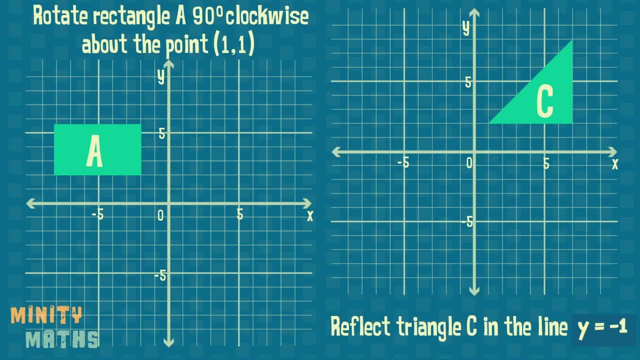 When drawing the new length part, you can now change the length of the new one, 거지 calidad, by using ones example. if you wouldn't mind, We can then reduce this value by adding more of them. democracy4win 10-30. 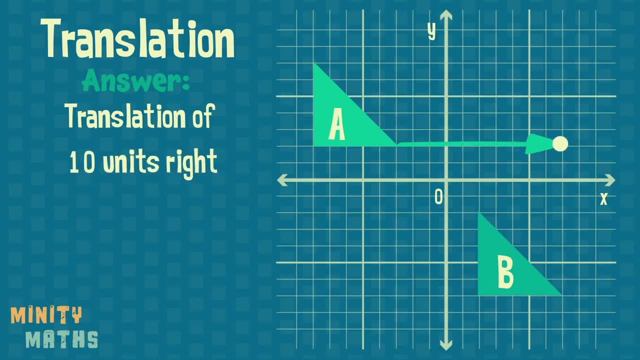 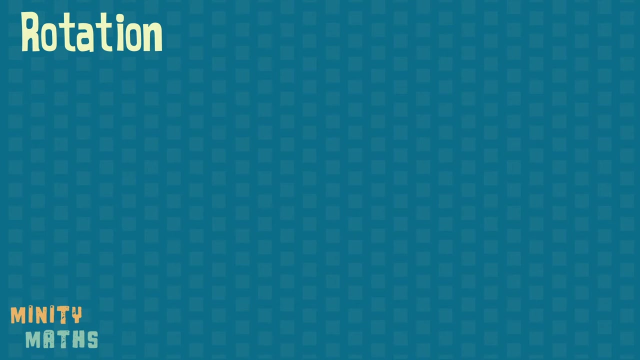 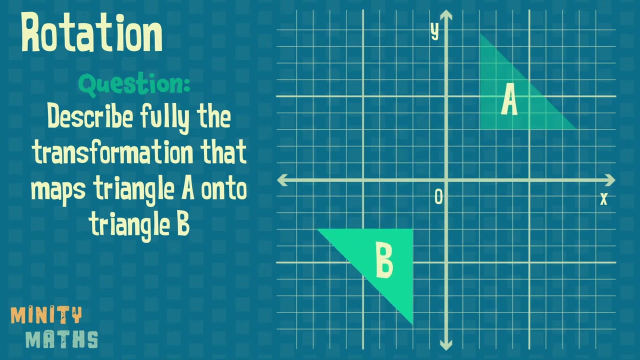 change vertically. Pick any vertex of the shape and use this to count how many units the shape has moved horizontally and vertically. We can also use vectors to describe translations. Rotation also changes the shape's position. To describe rotation, we must provide three details. 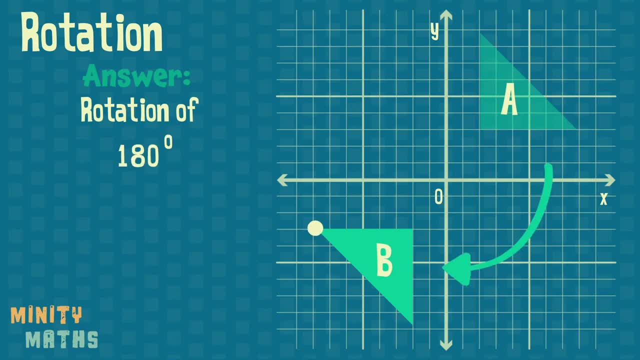 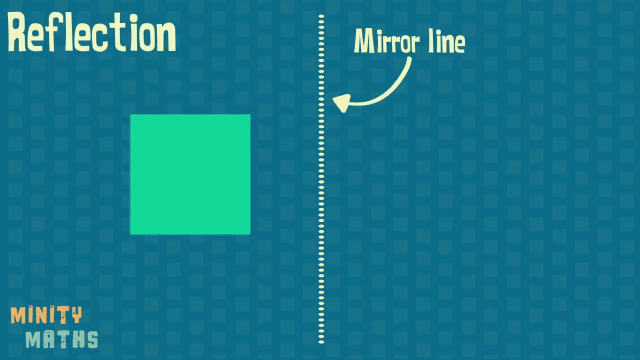 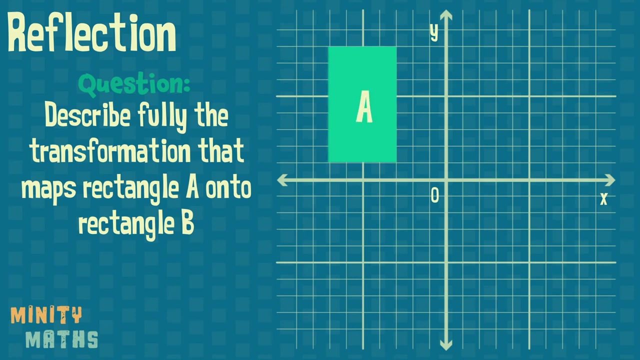 The angle of rotation, the direction and finally, the centre of rotation. You may find tracing paper helps with finding the point that the shape has been rotated around. Reflection changes the shape's position. Reflection of a shape can be described using only one detail, The equation of the line. 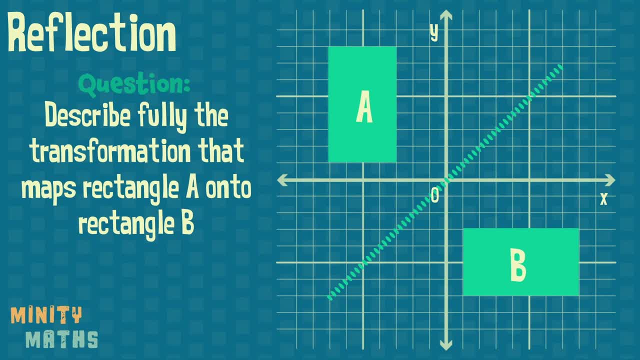 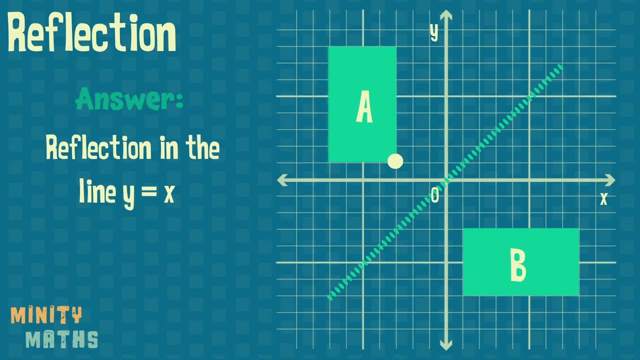 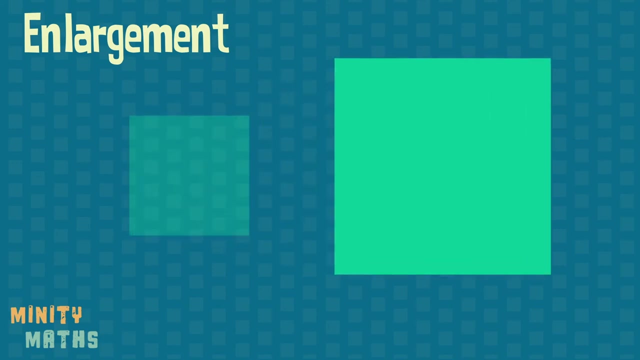 of reflection. It can help to think of this line as a mirror. Each vertex of the new shape will be an equal distance from the mirror line as each vertex of the original shape. Finally, enlargement changes the shape's size. To describe an enlargement, we need two details: The scale factor and the centre of enlargement. 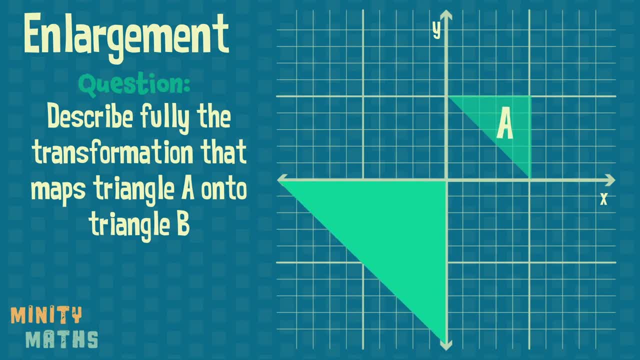 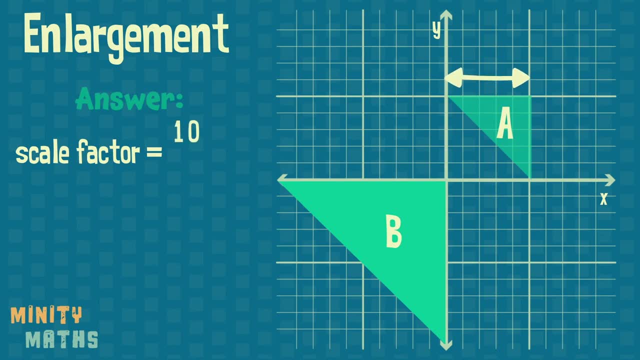 We can find the scale factor by measuring the length of one side of both the new and old shapes. We can then divide the new length by the old length. The new length is divided by one side. The new length is divided by the old length. 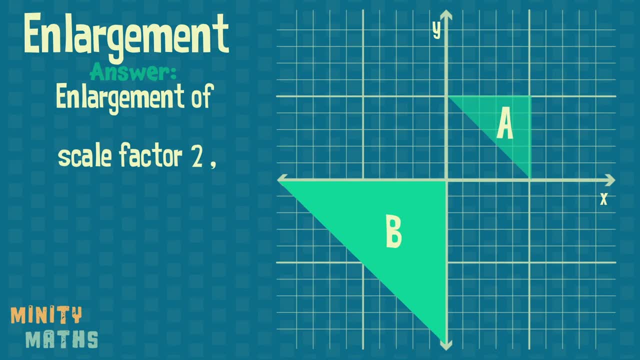 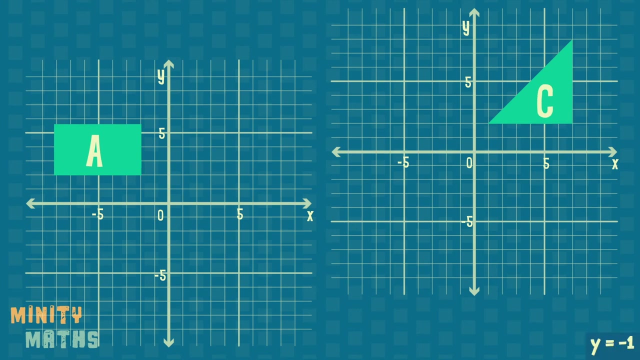 The new length is divided by the old length. To find the centre of enlargement, draw lines from the corresponding vertices of the new shape and old shape, extending them until they cross. The point at which they cross is the centre of enlargement. Have a go at these practice questions and pause the video while you figure them out. 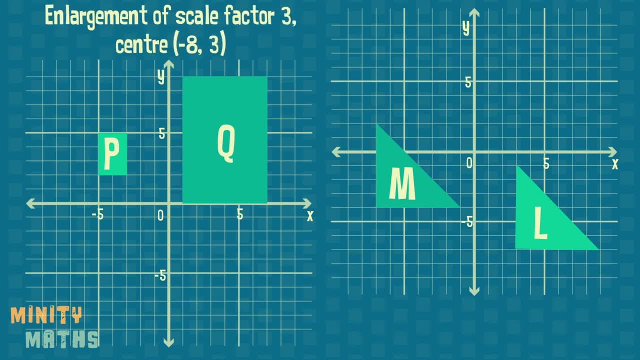 Thanks for watching. subscribe for more maths videos. 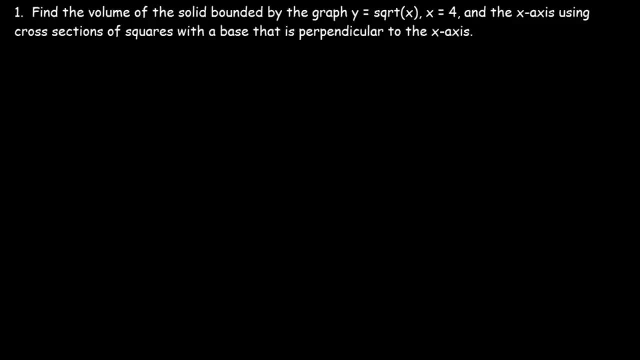 In this video, we are going to review how to find the volume of a solid using cross-sections. So there's two formulas that you need to be aware of. 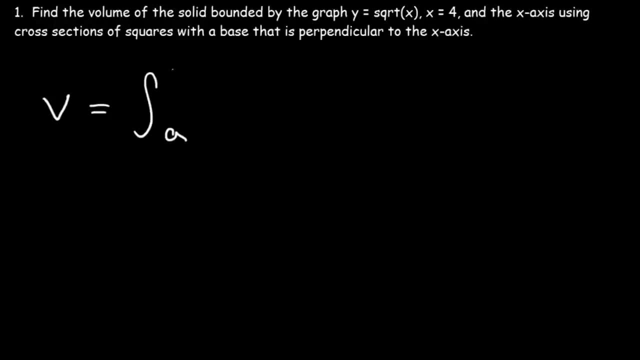 The volume can be found using this equation. It's the integration from A to B of the area function. 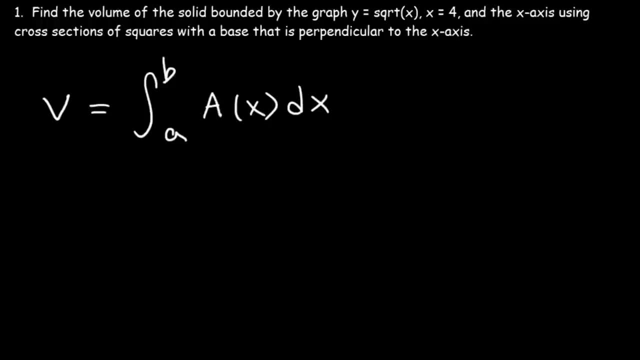 And if it's in terms of X, then the cross-section has to be perpendicular to the X-axis. 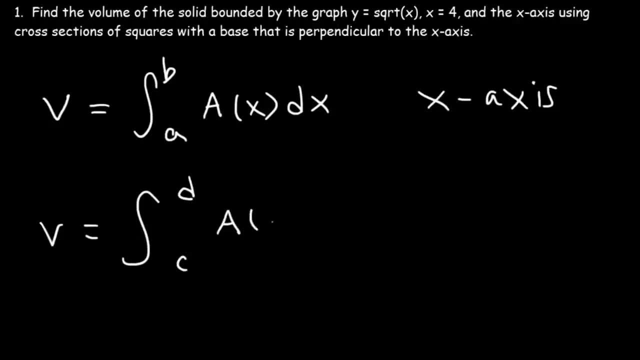 You can also use this equation. Where C and D are Y values. 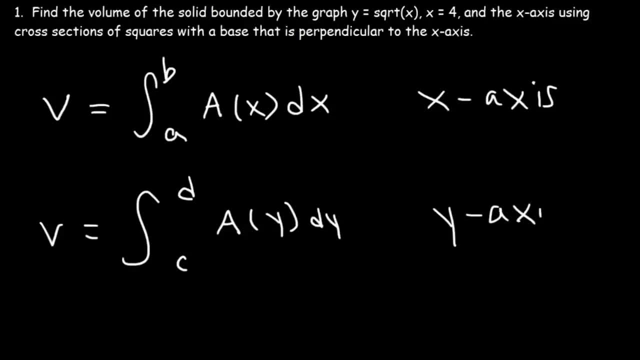 If it's in terms of Y, then the cross-section has to be perpendicular to the Y-axis. 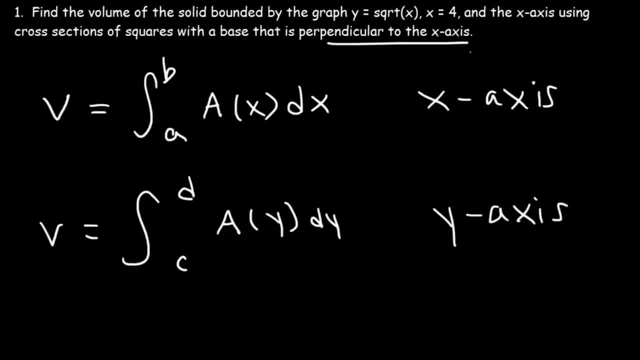 So for this problem, the cross-sections are perpendicular to the X-axis. Now let's go ahead and draw a graph. 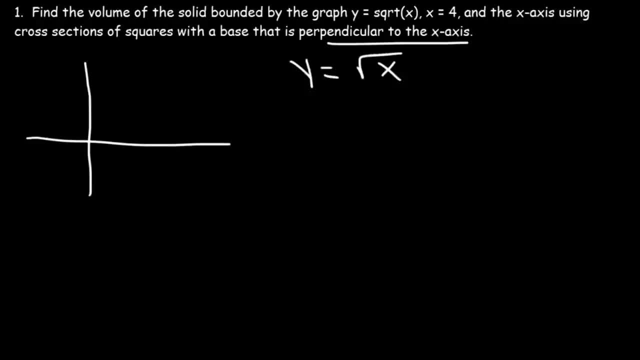 So Y is equal to the square root of X. And it's bounded by the X-axis. And the line X equals 4. 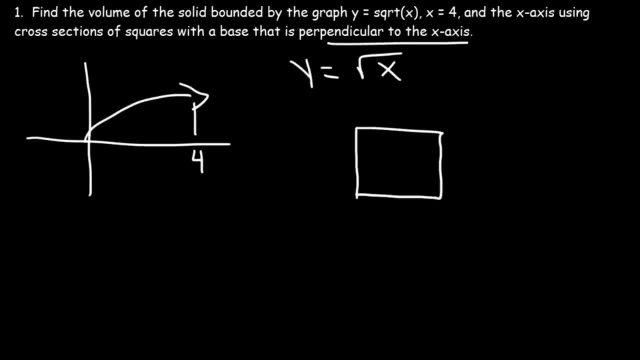 Now if we draw a square, the cross-sections are squares. The area of the square is basically side squared. And S is perpendicular to the X-axis. S represents the base of the cross-section. 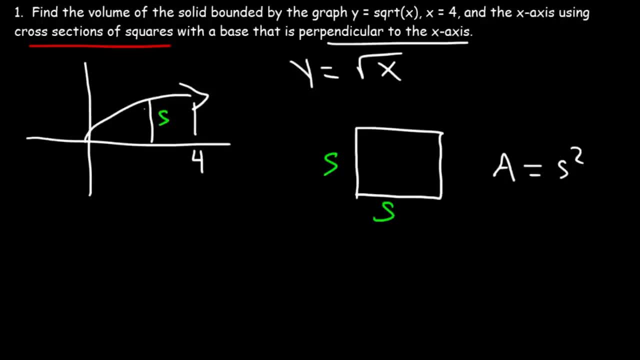 so notice that s is the same as y so the area which is s squared is also equal to y squared and y is the square root of x our goal is to get the area function in terms of x 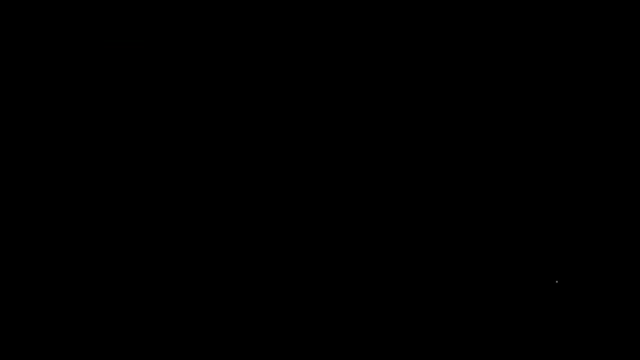 so a of x is equal to x so if we integrate it from a to b this will give us the volume so we're going to integrate it from